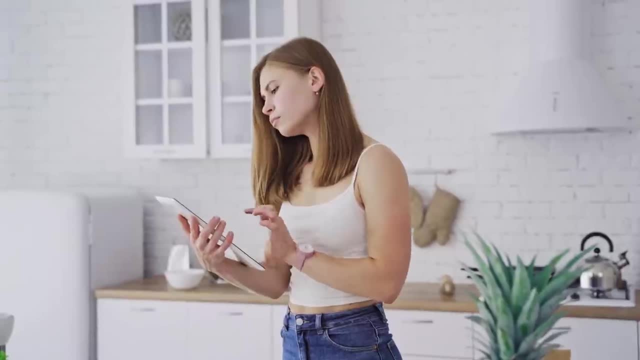 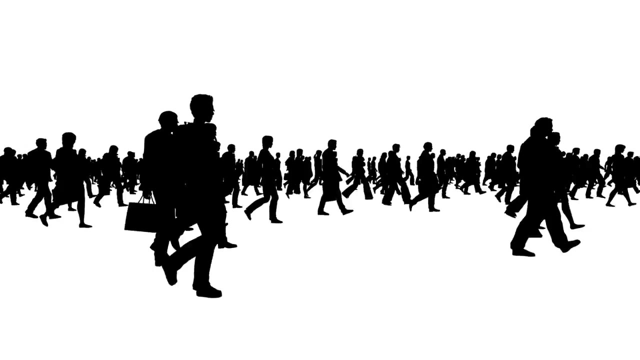 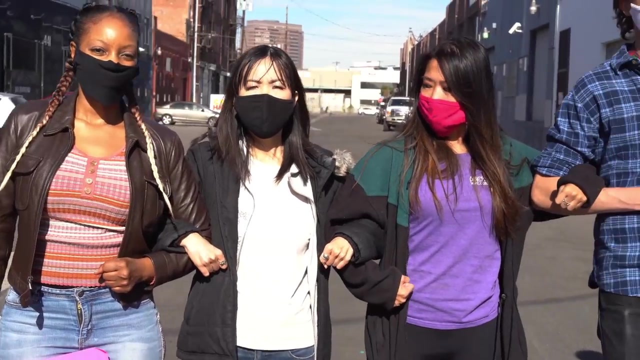 People pointed out that it's not just racists that want to know the demographics of a location. People of different races like to know where to live so they can be near types of restaurants they like, stores and different festivals, things like that. To me that argument made sense. so a few months back we did a video on the most Asian states in the US. 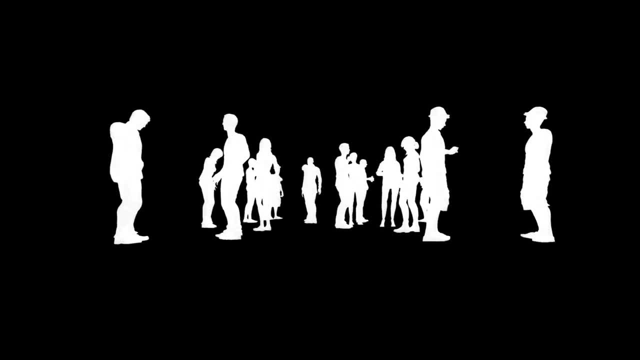 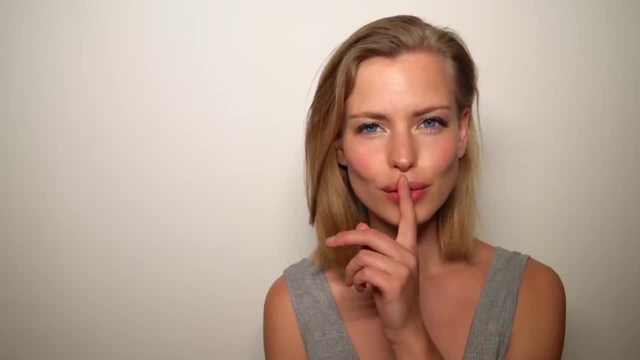 and then later on we did the most Hispanic states. Today we are doing the whitest states. I mean, it's kind of only fair. We're going to look at the percentage of the population that is considered white. We'll also look at what European people settled in that area first, 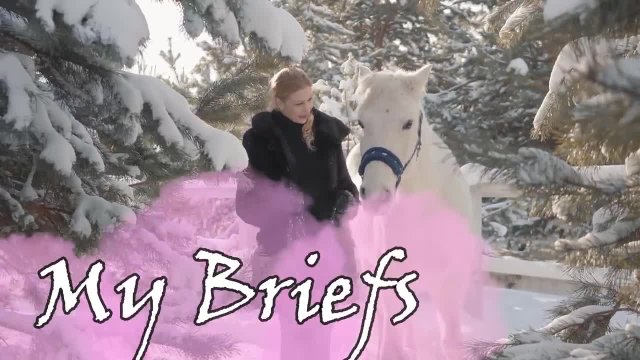 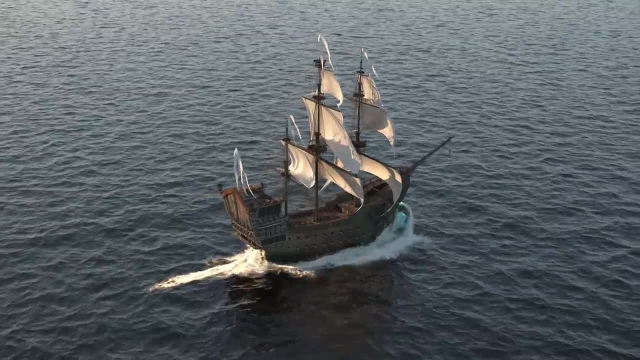 and this is all according to the US Census. And now a brief overview: Around 1565, the Spanish showed up in St Augustine, Florida. Then, of course, the Mayflowers. The Mayflower showed up on November 11th 1620. 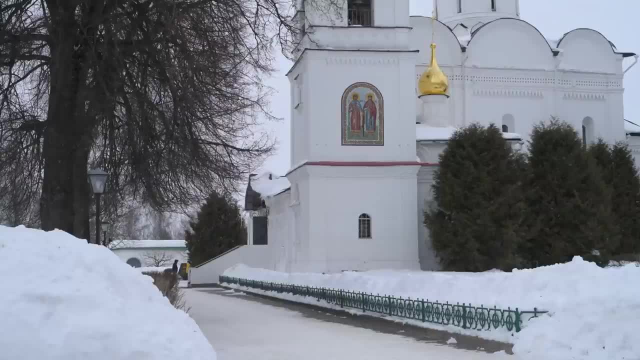 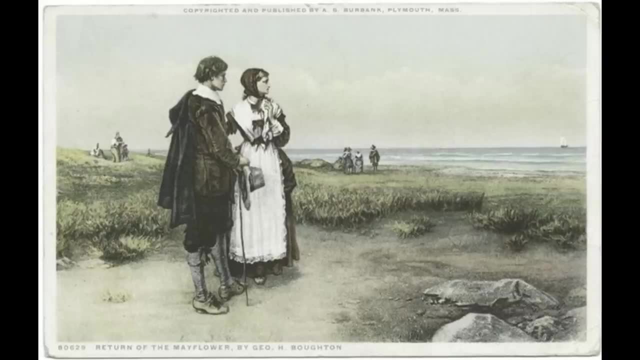 Now there's a whole bunch of other stories with explorers and Russians in Alaska and all that other good stuff, but the two main things in the history book of North American colonization is the Mayflower and then the Spanish down in St Augustine. 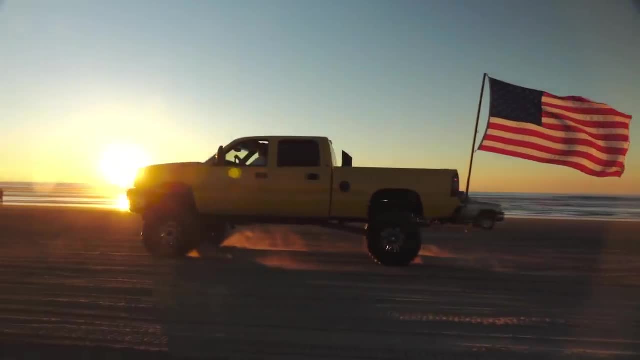 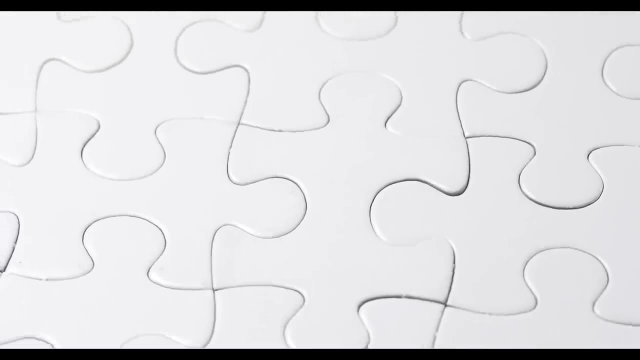 Whatever the case may be, or the story may be, white people took over, and what is now? the United States has been predominantly white ever since. Today, we're going to look at 10 states whose percentages haven't changed much since the 1700s. 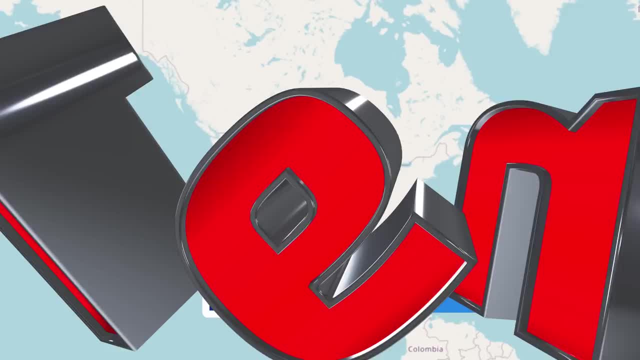 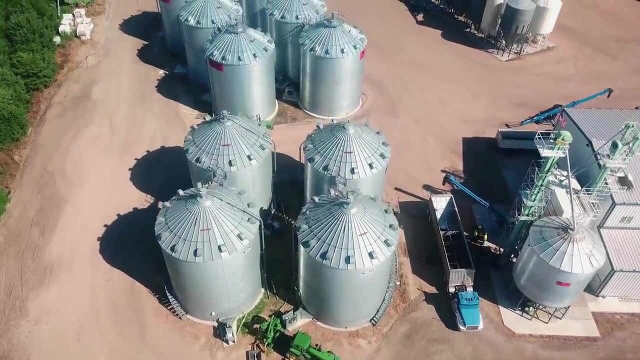 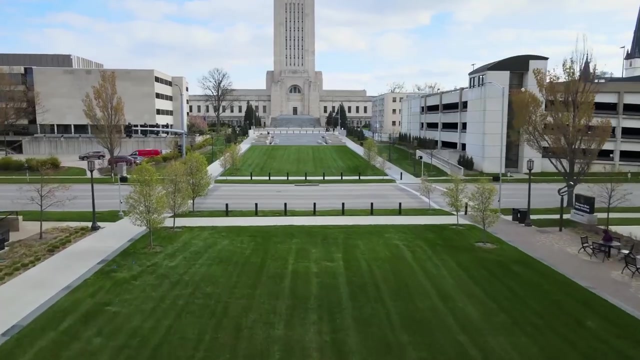 Got it, Get it Good. Let's take a look. Number 10, Nebraska. Nebraska is extremely white, and they start our list off. By the 1870s, Nebraska's European immigrant population was at its peak and about 25% of the state's residents were born in a foreign country. 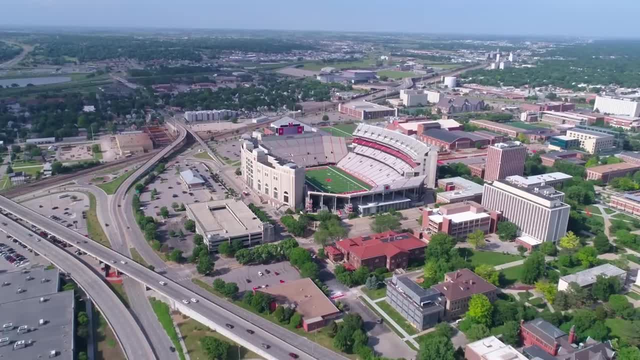 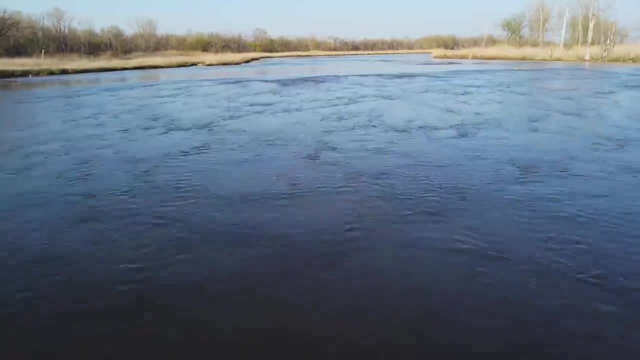 Danes, Swedes, Irish, Germans and Czechs figured predominantly among the early newcomers to Nebraska. If you need more proof that Nebraska is extremely white, take this into consideration. The number one male name in Nebraska is Oliver, followed by Henry and Liam. 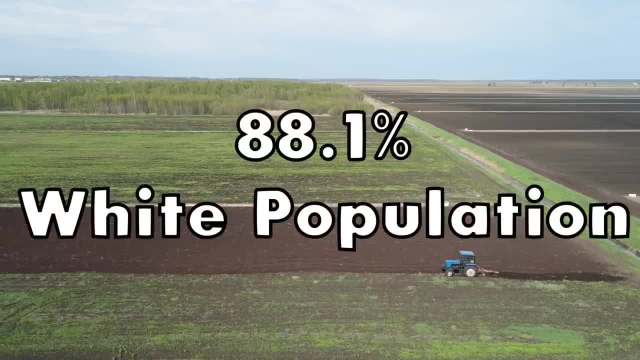 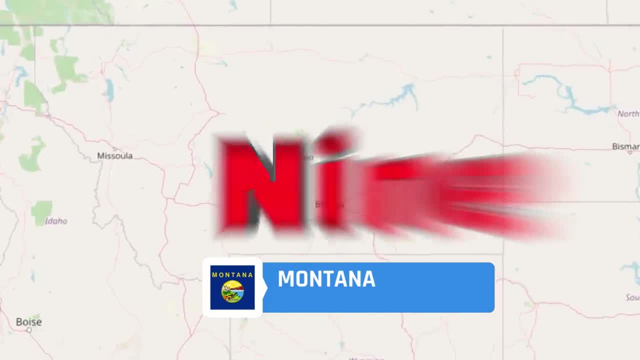 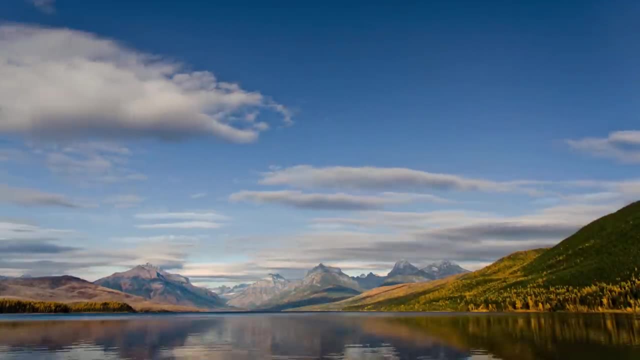 Number four is Theodore. 88.1% of Nebraska's population is white. Number nine: Montana. Coming in strong with the blonde hair, blue eyes crowd, you have Montana, Originally Italians and Germans settled in Fergus and Park counties. Many Germans came from North Dakota and Canada and a lot of the cattlemen that landed in Montana were mostly English and Scottish. Now, the dynamic back then was the English and the Scottish basically worked the cattle, but the owners were typically German. 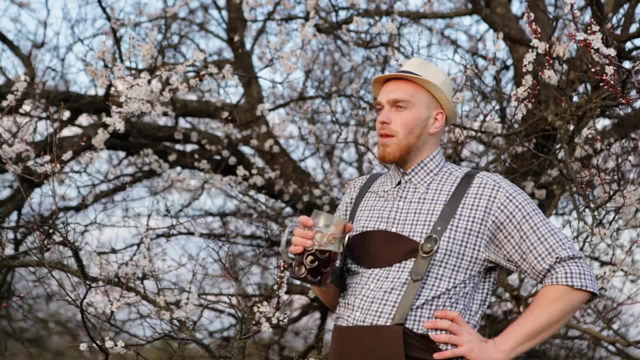 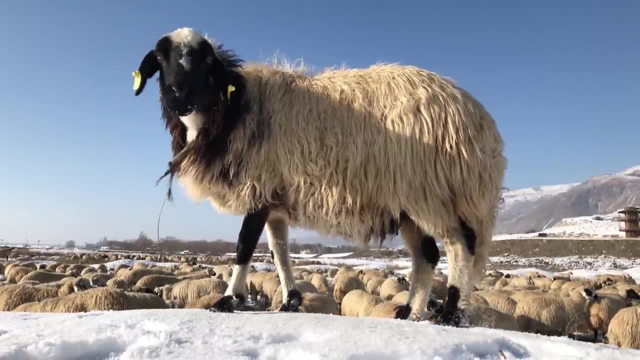 Now they did have sheepmen. Sheepmen normally weren't okay back in the day. The cattle guys didn't really like them. but there were a lot of them in Montana and they were from the British Isles. That's how Montana became the Montana we know today. 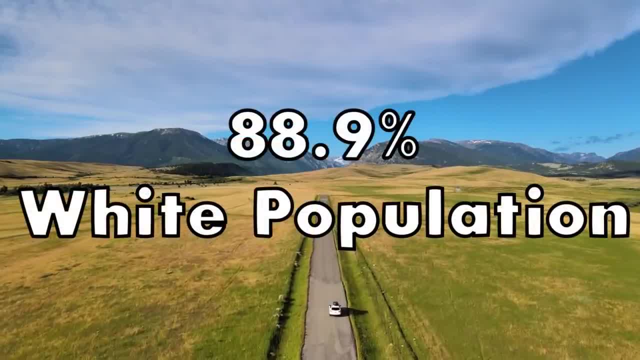 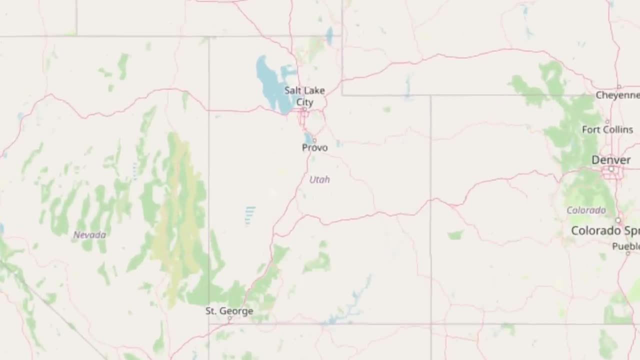 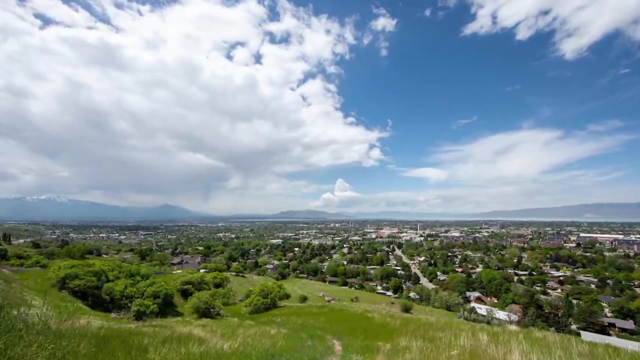 Number eight: Utah. If you didn't know, Utah was mostly white. you've never been in a Mormon temple. Mormons make up about 70% of the Utah population and they have a history of being so white they think Malcolm X is a member of the X-Men. 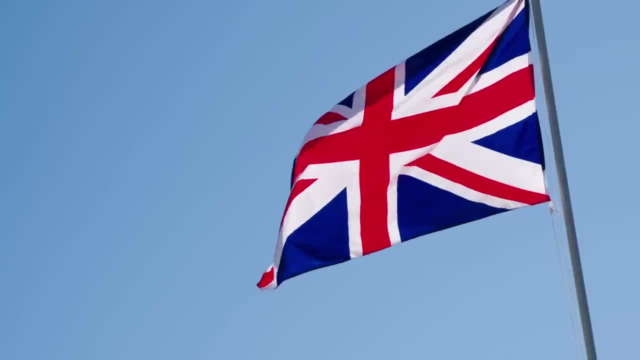 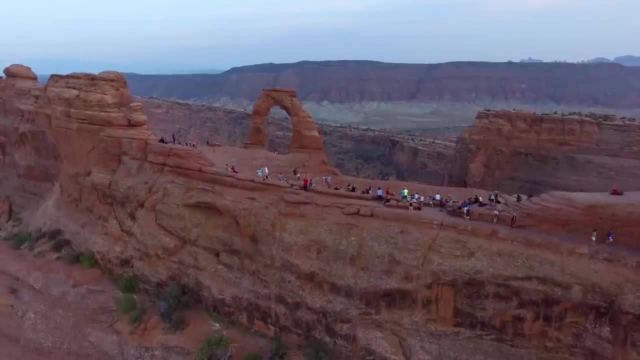 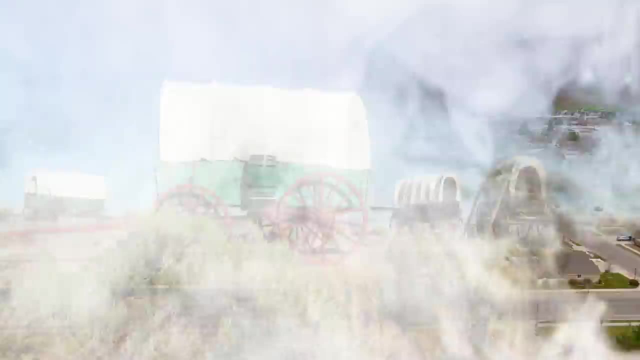 In the early days, Spanish explorers and French, Canadian, British and Canadian fur traders had briefly stomped around Utah before 1847, but it was that year that the Mormon immigrants from Britain, Canada, Denmark and Norway were part of the Mormon exodus from Illinois and became the 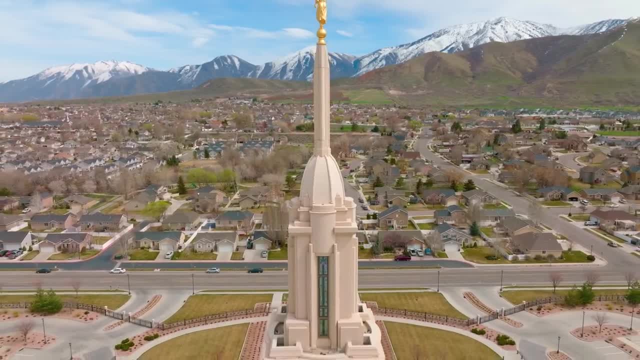 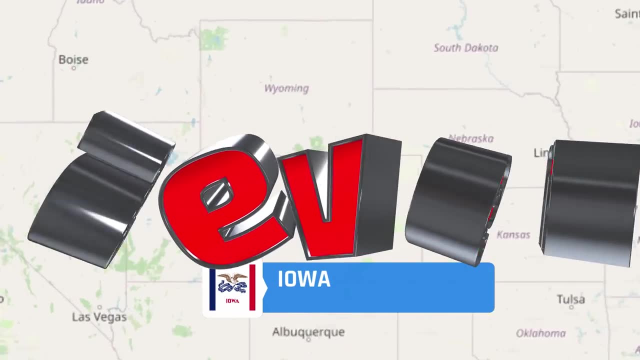 first non-Native Americans to settle in the future beehive state. 90.6% of Utah's population is considered white. Number seven: Iowa. If you didn't know Iowa's very white. You've never been to a county fair in Iowa. 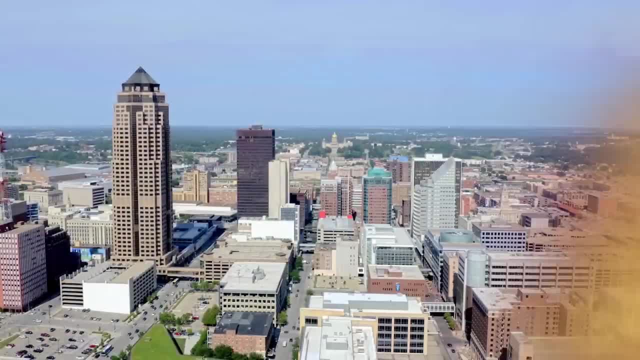 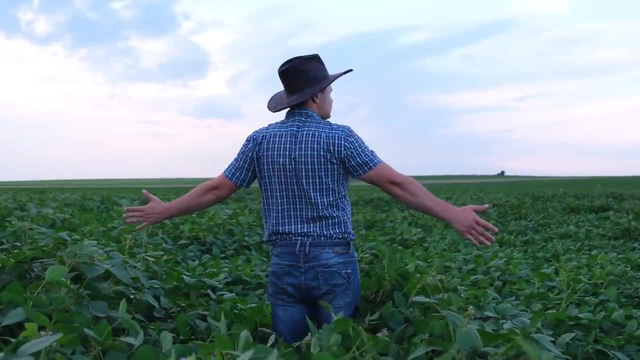 Before I started doing the research for this video, I honestly thought it was gonna be number one. I've been to Iowa a few times and it is probably the whitest state I've ever seen. At least that was my opinion. The numbers don't match up with my opinion. 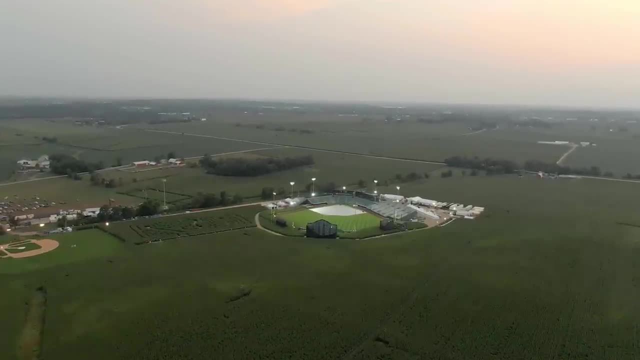 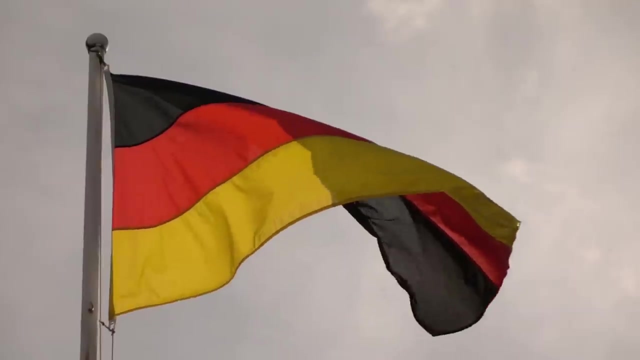 So here they are at number seven. Back in the early days, like the 1840s, a majority of the settlers that came to Iowa came from the Scandinavian countries. Some were Dutch, German, Irish, Scots and Welsh. New Englanders started showing up that same time. 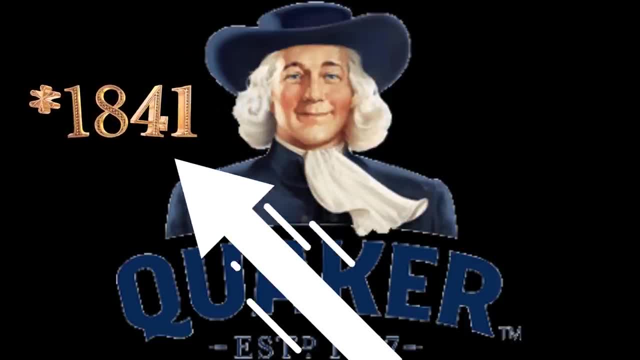 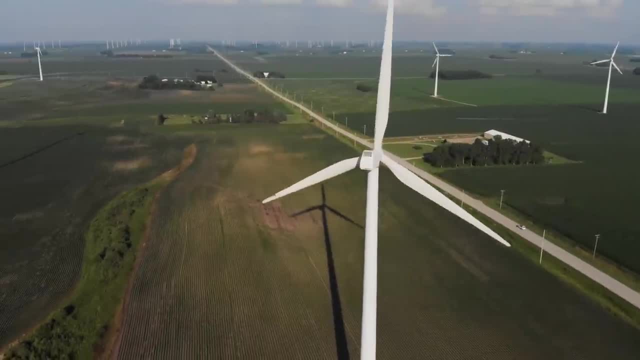 along with Quakers in 1941, and then the Mormons started showing up around 1846.. Yes, Iowa has a good-sized population of Mormons as well. Nothing near what Utah has, but it's up there. These days, 90.6% of Iowa's population is white. 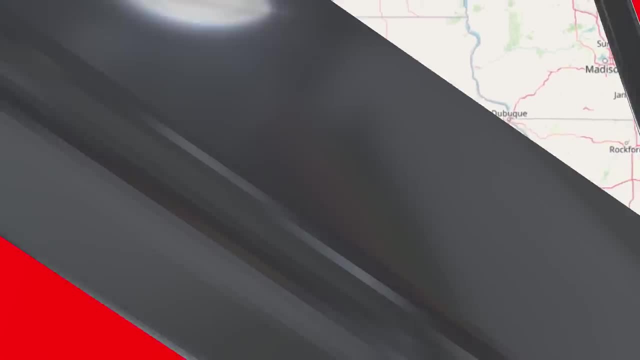 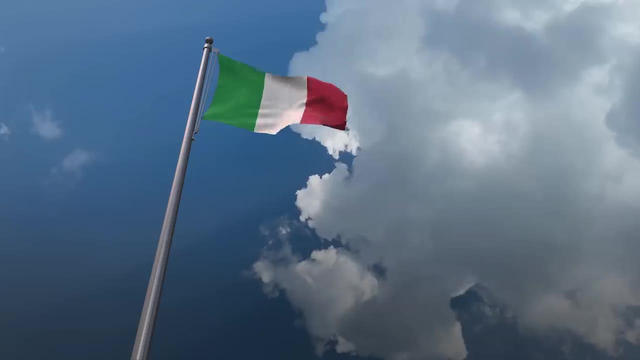 These days, 90.6% of Iowa's population is white. These days, 90.6% of Iowa's population is white. Number six: Wyoming. There were six groups that made up the early immigrant settlers of Wyoming: The British, the Germans, Italians, Basque. and the Greeks showed up here In 1870, immigrants from the British Isles represented about 1 5th of Wyoming's territorial population and over 1 1⁄2 the foreign-born population. So the Brits came in strong. 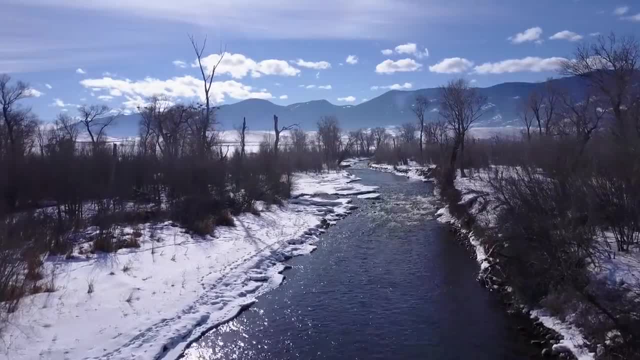 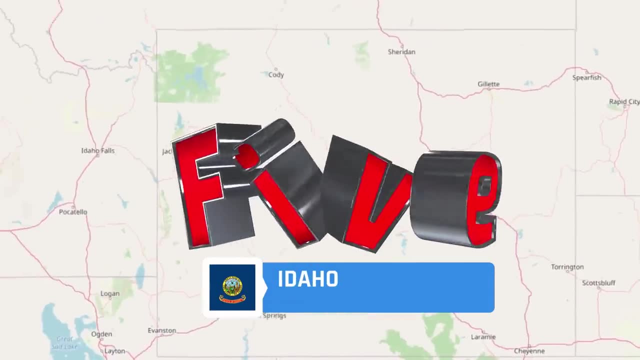 In the last few decades, Wyoming's become very popular with just about everyone, But these days 92.5% of their population are identified as white. Number five: Idaho. Idaho has quite the reputation for being very white. It has always been that way. In the late 19th and early 20th century a large majority of the settlers were English, many before statehood. This seemed like a really great place to them because there wasn't much government Back in those days. most of the English from jolly old England. 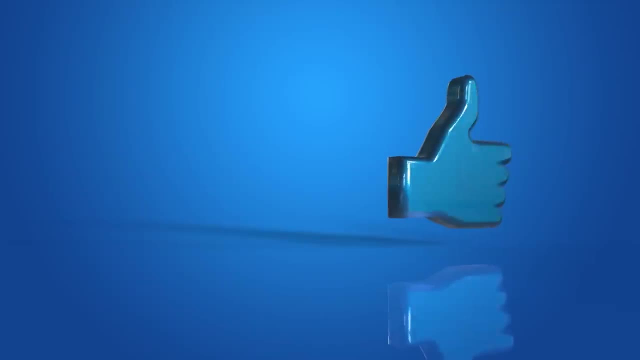 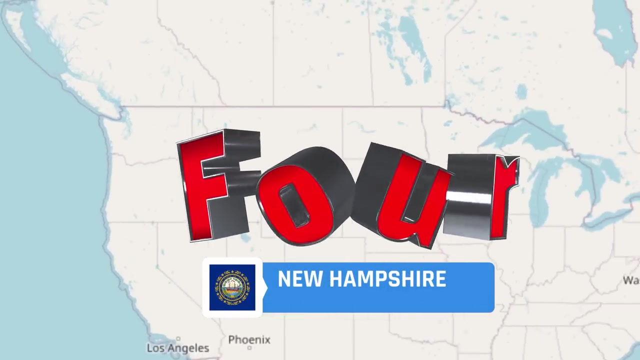 were being taxed to death and a place with next to no government seemed like a great place to live. 93% of Idaho's population is white. Number four, New Hampshire. This is another state that should be no surprise to anyone that's ever been to New Hampshire. If you live there you already know. I mean, we're talking about a state where the people consider Taco Bell diversity. New Hampshire, being part of New England, obviously goes back to the colonial days And at the time it was mostly British residents. in the area that would eventually become New Hampshire, But in 1799, they started being joined there by a lot of Scottish and Irish immigrants, And in 1799, New Hampshire- they became part of the French-Canadian population. What's strange is for a long time. 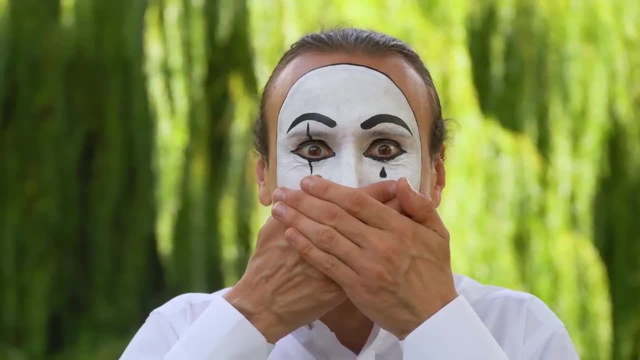 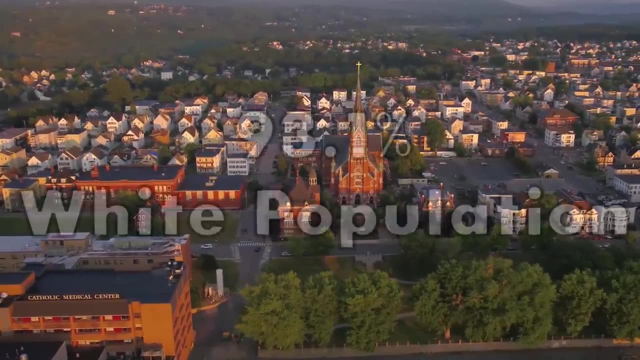 they had a lot of French-Canadians living in New Hampshire and sometimes you could find little bits and pieces of that culture in New Hampshire. They came down for the textile mills from Quebec and a lot of them stayed back in the day. 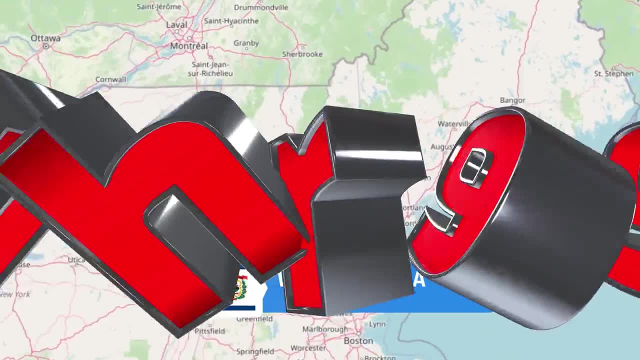 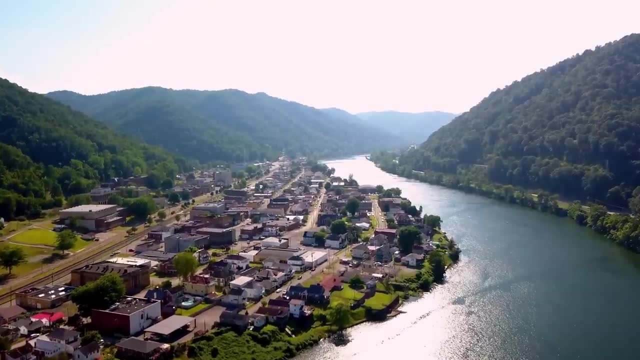 These days, 93.1% of New Hampshire's population is considered white. Number three: West Virginia. West Virginia is kind of strange. I thought they would be a little bit higher as in the percentage, because, unlike most cities in the United States, 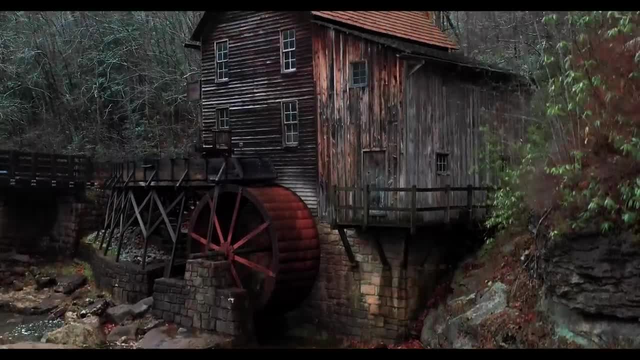 West Virginia is a little bit more diverse And if you look outside the cities and some of the rural areas, the mountains and the hollers especially, there is like zero diversity. So I'm actually a little surprised they're number three on this list. 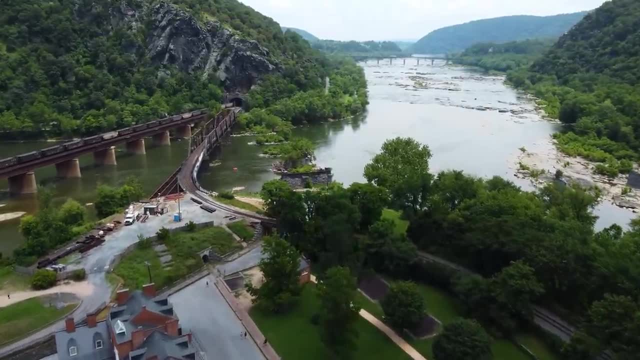 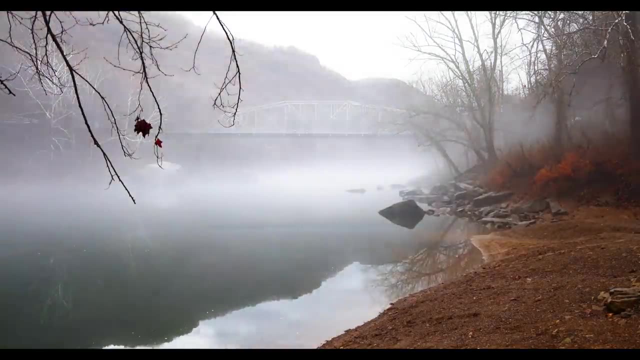 The settlement of present day West Virginia began in the mid 1700s, when Scottish, Irish and German settlers from Pennsylvania came to the area that is now Berkeley and Greenbrier Counties. The Scottish and Irish cultures really soaked into the West Virginia land. 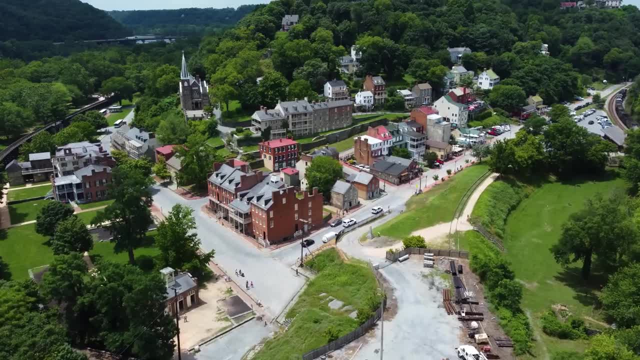 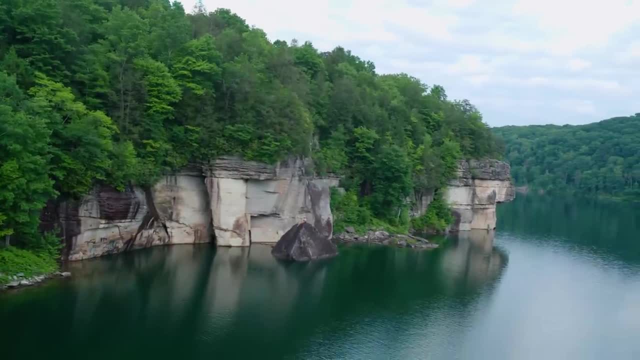 A lot of the folk music in this part of the country is heavy with Scottish and Irish folk music And it's a lot of folk influence. These days, 93.5% of West Virginia's population is identified as white. Number two, Vermont. 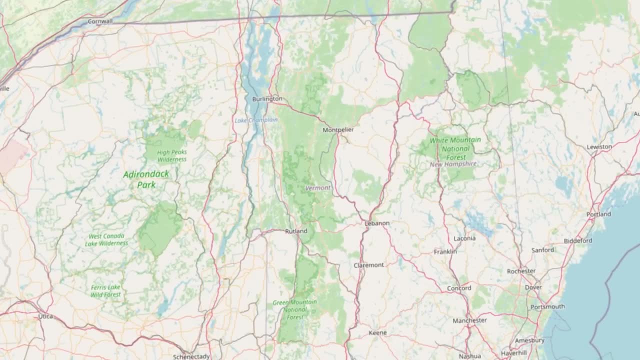 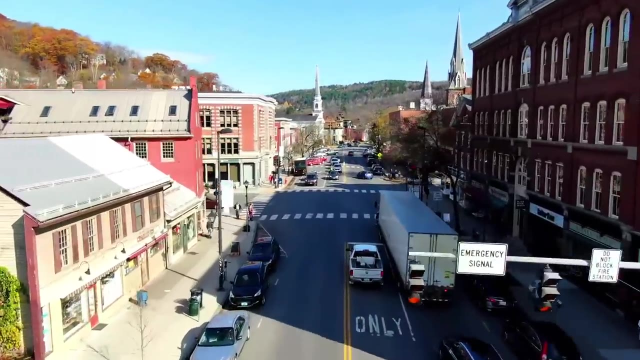 Remember everything I said about New Hampshire? Well, it's the same in Vermont. It always seems to be that way. I mean they're right next to each other and they always seem to show up really close on lists. You look at their crime stats. you look at their school grades, their economies, they're always right next to each other on whatever stat we're looking at. Like New Hampshire, the place was settled with the English, the Irish and the Scottish eventually, And they also had a fair share of people coming down.